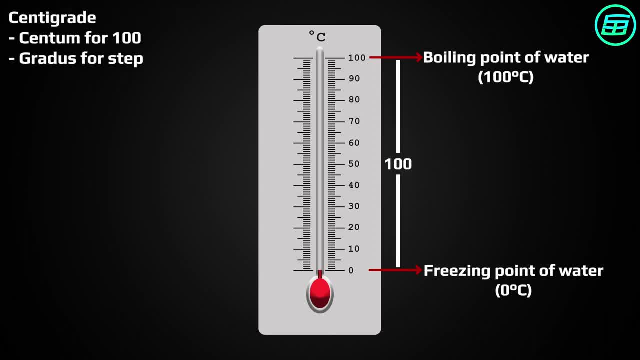 It was called centigrade, From the Latin centum for one hundred and gradus for step. Now we know it as the Celsius scale. In 1848, William Thompson, also known as Lord Kelvin, developed a temperature scale based on absolute zero. 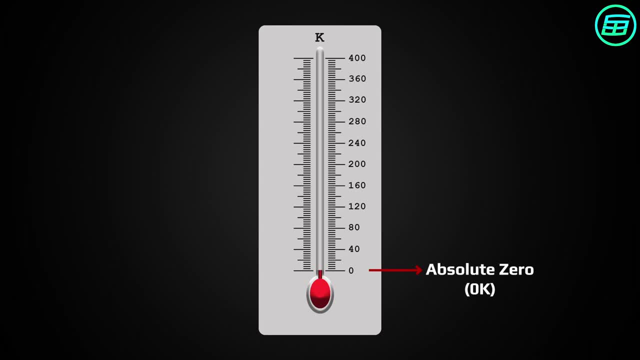 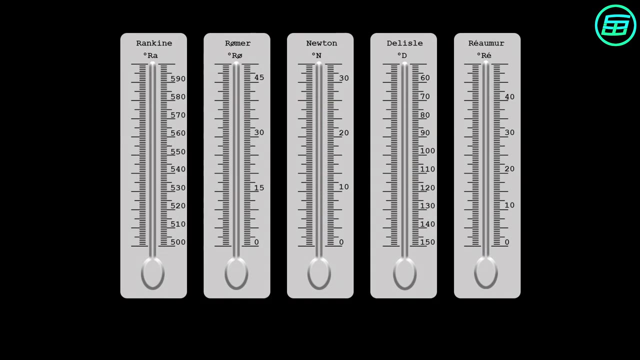 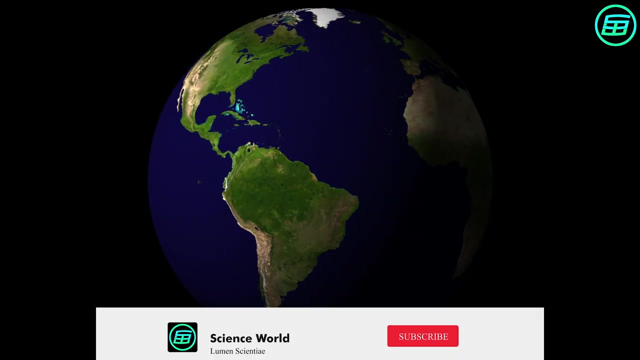 theoretically the lowest possible temperature On the Kelvin scale. pure water freezes at 273.15 Kelvin and boils at 373.15.. Other scales were proposed in the past but never came into widespread use. Only a few countries still use Fahrenheit as their official scale. 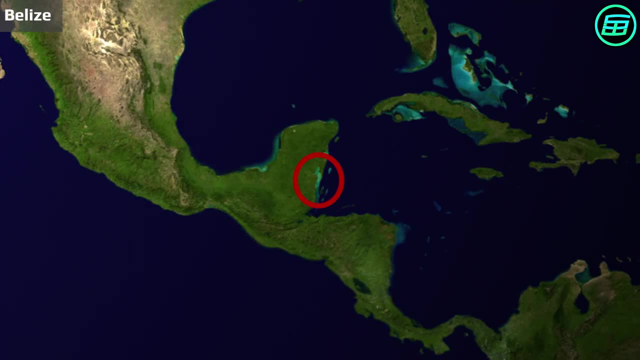 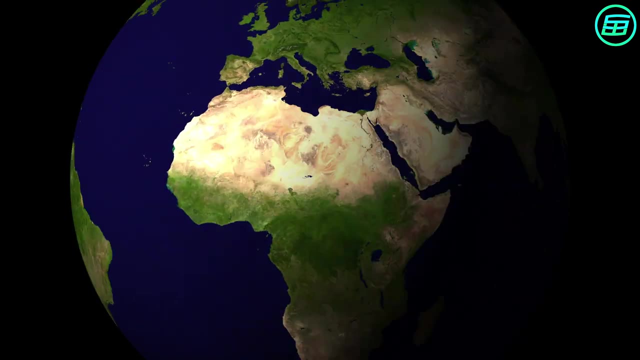 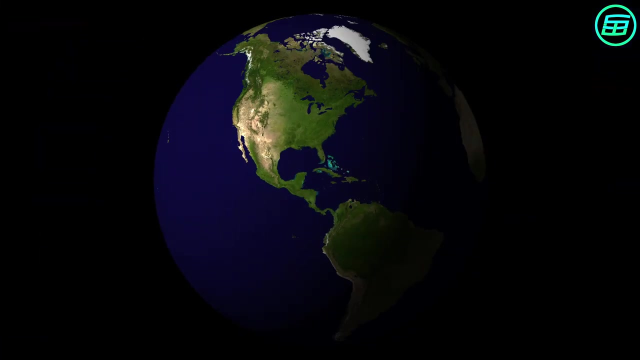 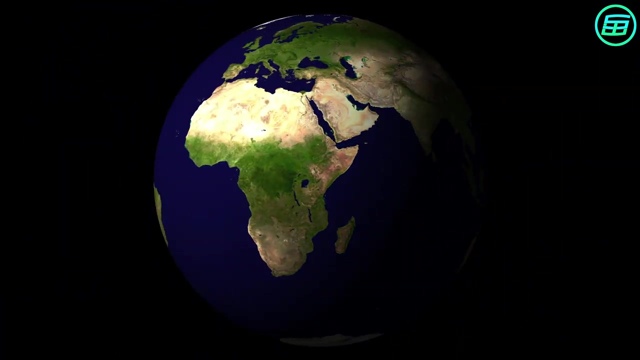 The United States, Belize, Palau, France, the Bahamas and the Cayman Islands. Fahrenheit is still sometimes used in Canada, although Celsius is more common and is the official Canadian temperature scale. In the rest of the world, the Celsius scale is used. 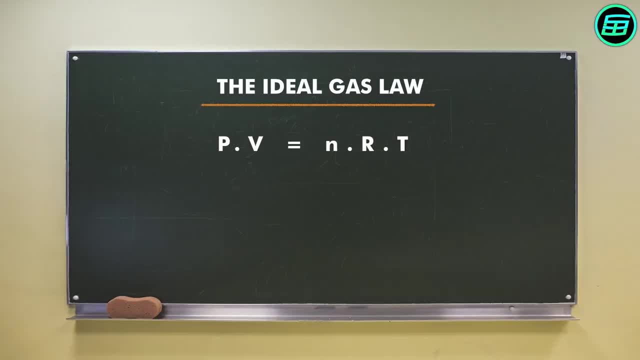 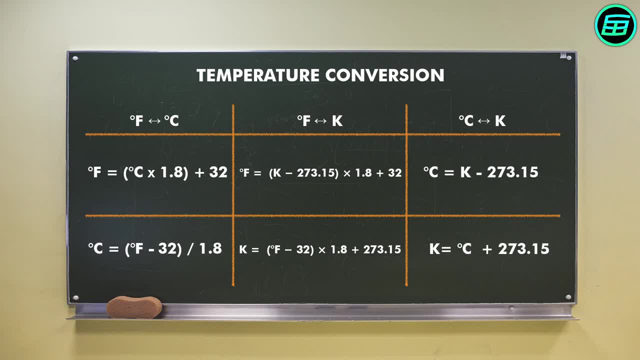 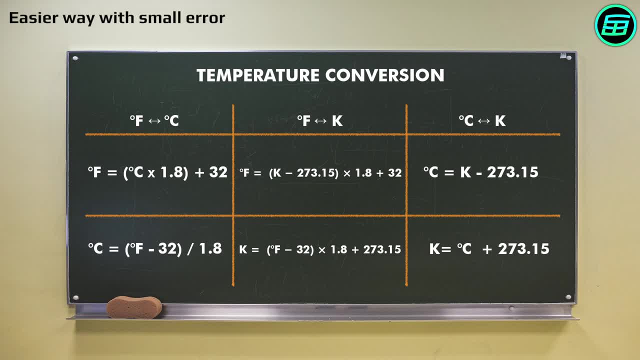 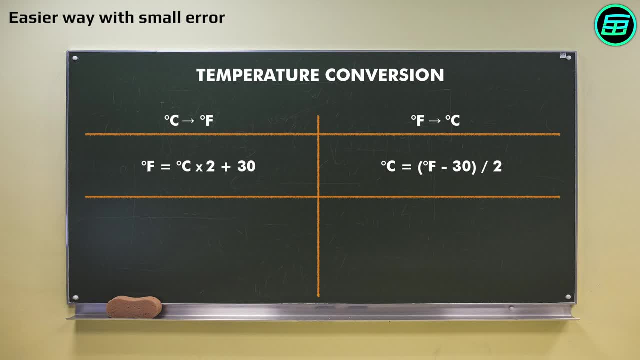 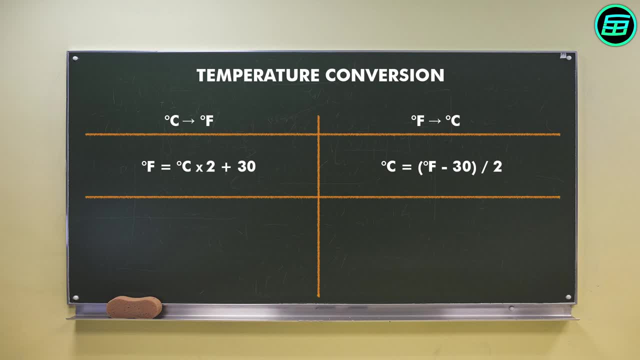 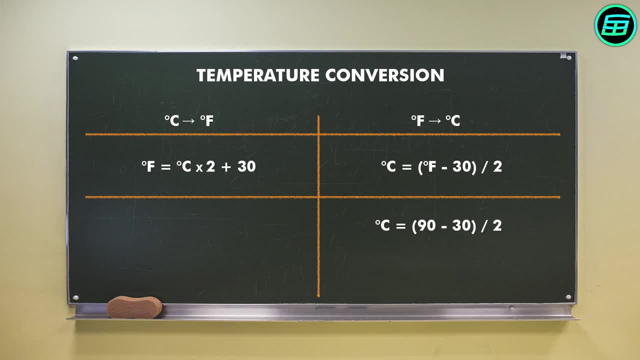 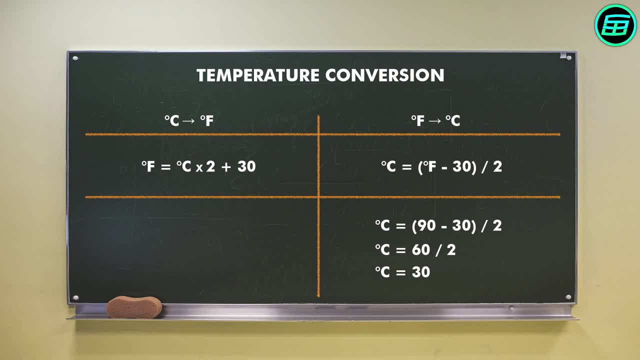 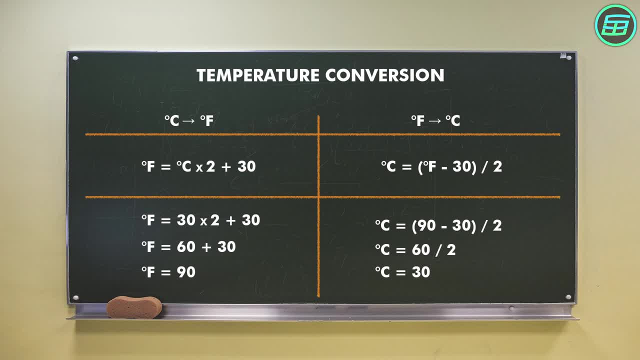 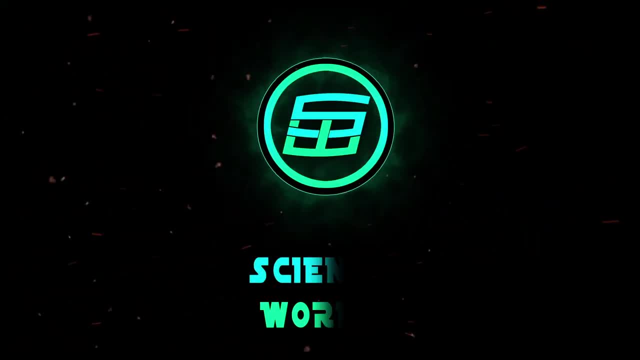 In order to convert temperatures in one scale to another. these formulas are called Kelvin scales. 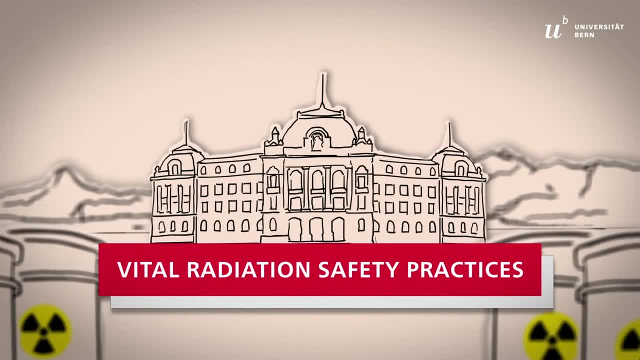 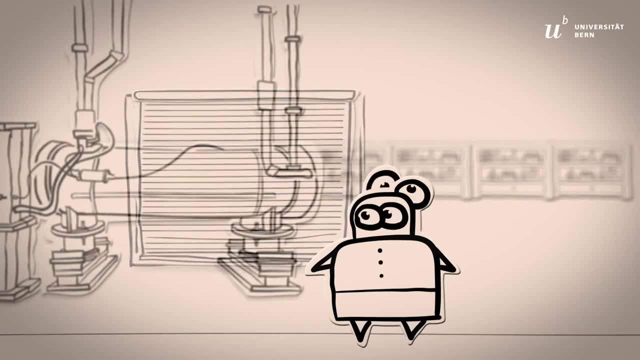 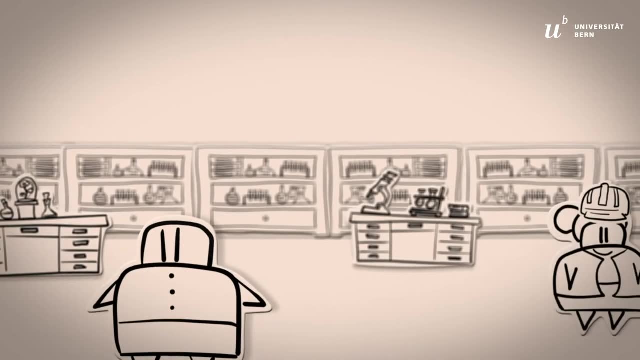 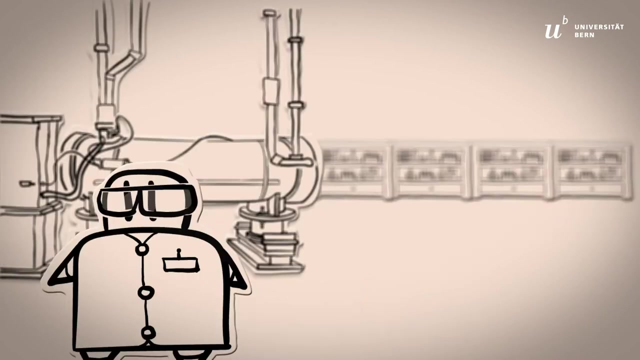 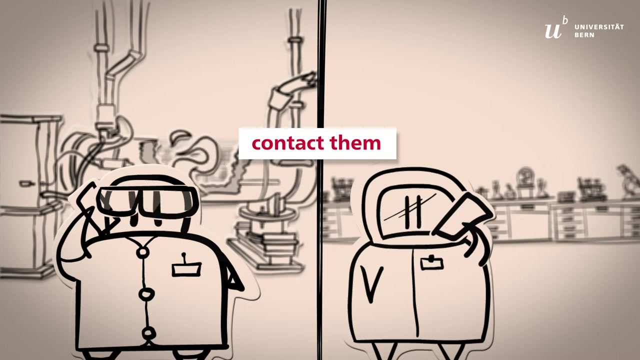 Vital Radiation Safety Practices. Working with radioactive sources comes with certain risks. You can minimize the risks at our university by following these safety practices First. you should know that besides your supervisor, there is a radiation safety officer in your department. Before any activity with radioactive sources you must contact them for a risk assessment and instructions. 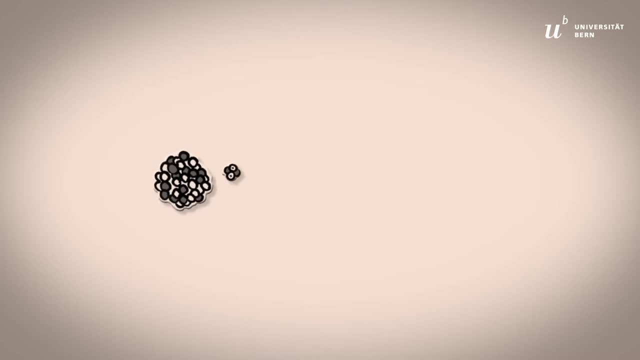 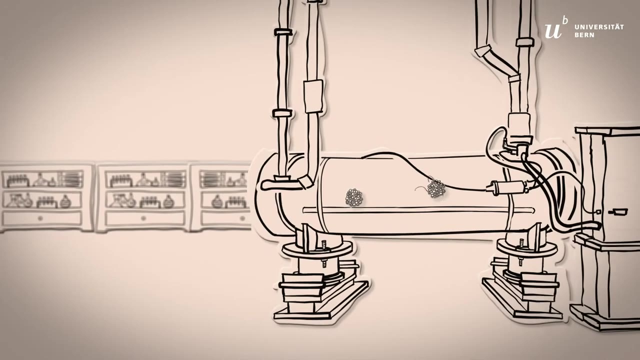 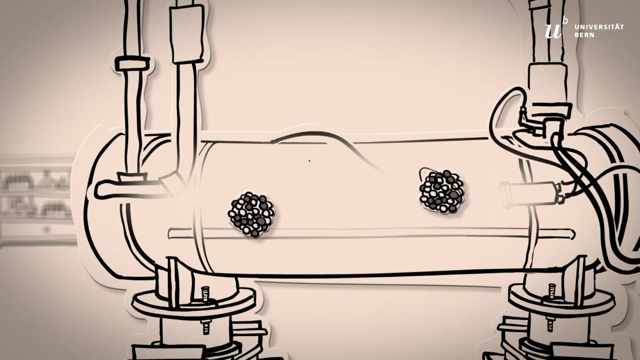 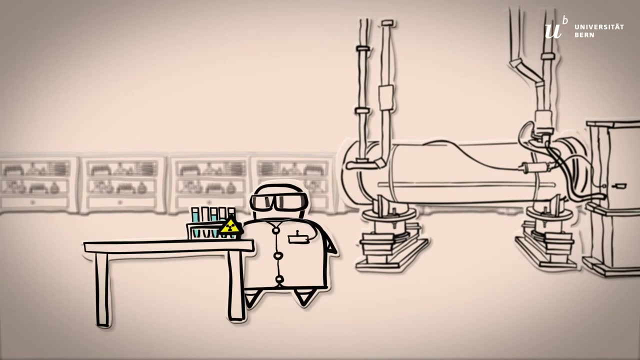 Radioactive sources emit ionizing radiation in the form of alpha and beta particles, as well as gamma rays. They are divided into sealed and unsealed sources. Sealed sources are designed to prevent the release of radioactive substances. Unsealed radioactive sources are not encapsulated and pose the risk of contamination. 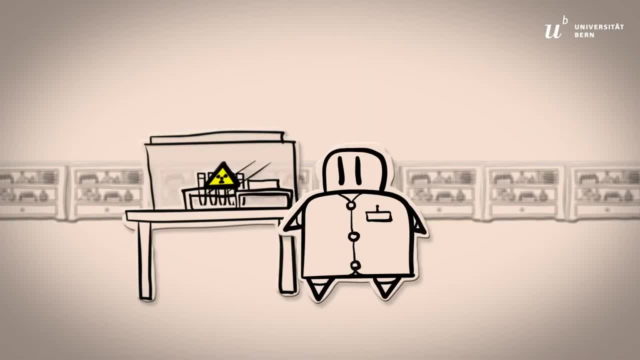 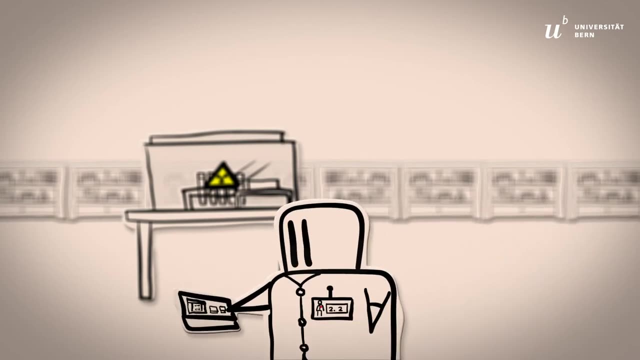 Exposure to ionizing radiation can result in severe health problems, such as burnt tissues and cancer. Hence exposure limits have been established to reduce the risk. The health effects of radiation on the human body are measured in sievert using film badges or dosimeters. 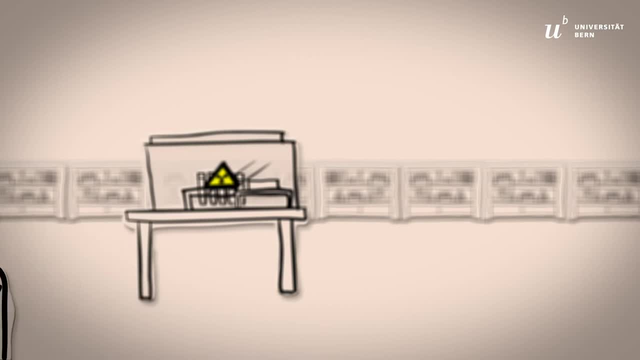 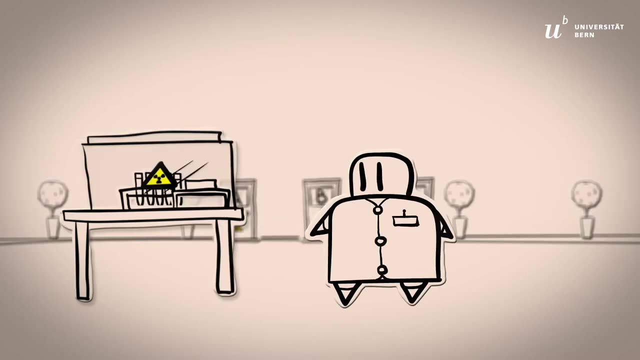 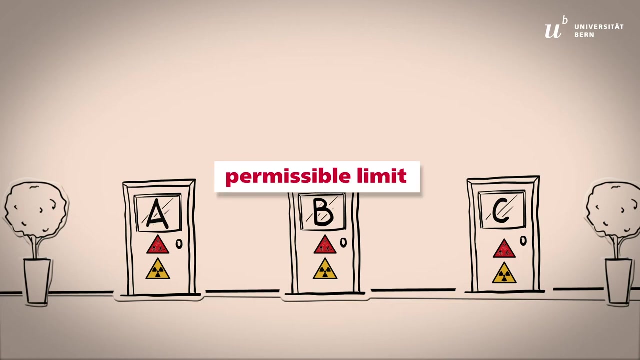 For occupationally exposed persons, the effective dose must not exceed the limit of 20 millisievert per calendar year. To prevent accidental exposure, you must adhere to the following safety measures when working with radioactive sources. Laboratories for working with radioactive sources are classified into three types, based on the permissible limit and the radioactivity of the sources handled. 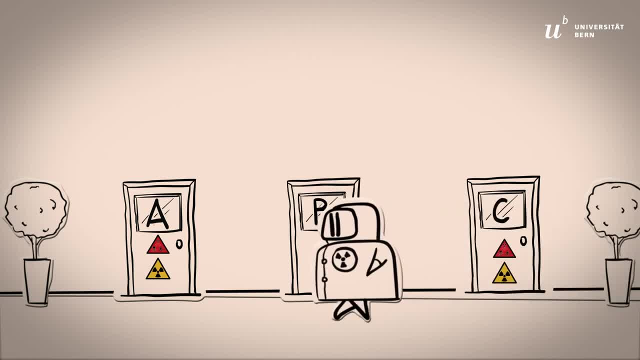 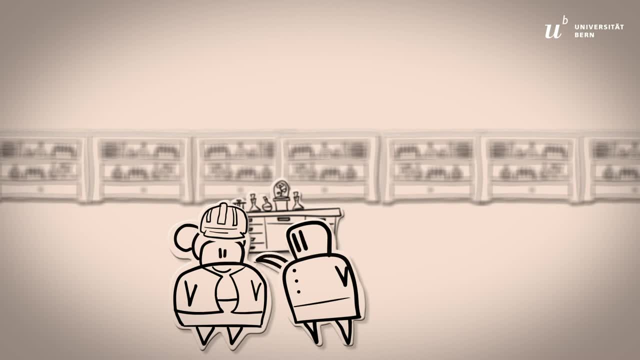 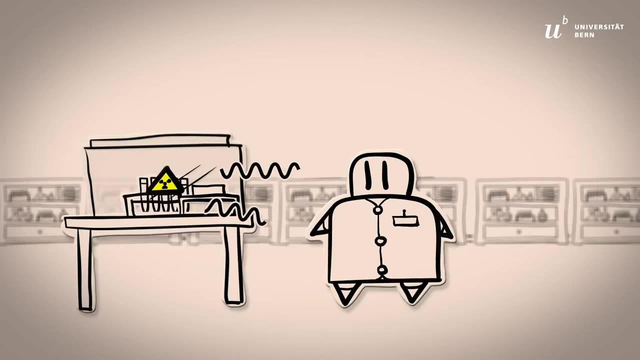 They are marked with radiation hazard symbols and access is only granted by the radiation safety officer. Contact your supervisor for instructions about what personal protective equipment you need and how to properly wear it To keep exposure to radiation as low as reasonably achievable limit your exposure time.